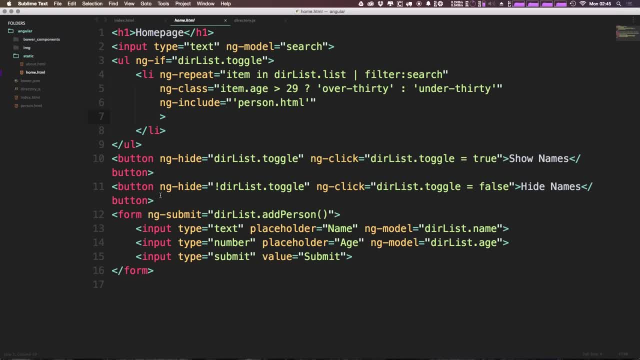 directives in your view already, Even if I said you don't realize them, they might be hiding in plain sight. We have ng-click, ng-hide, ng-class, ng-repeat, ng-if. These are all directives, And they are all directives in a specific form of a directive. 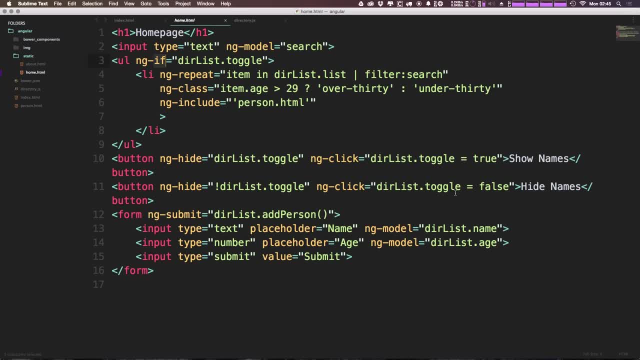 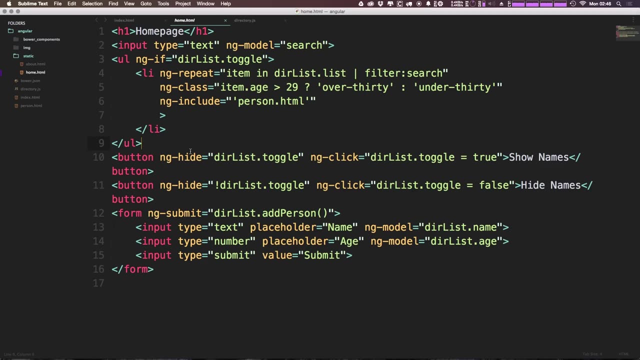 They are the directive that is being declared as an attribute on an element. So these are all being declared as an ng-hide attribute on a button or an ng-repeat on a list item. But directives can also be used in the form of actual elements, So you can write a directive. 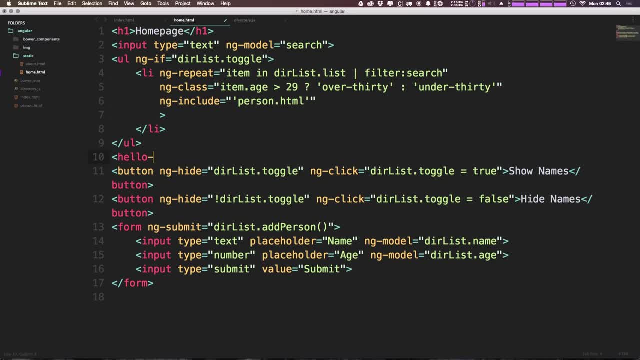 that looks like something like hello world, Just like you would any other HTML, And this can be past attributes. It can contain other custom elements. There's a lot of stuff here. You can also define a directive via a comment or even a class. 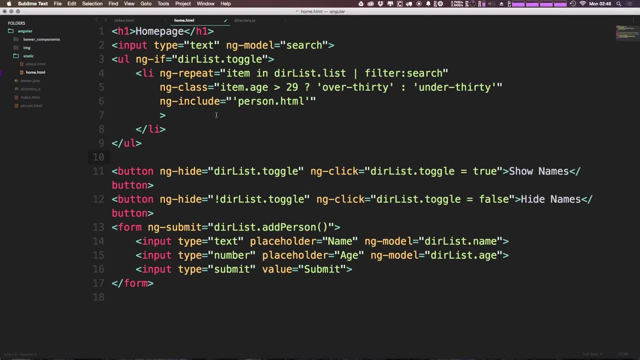 Now they do say that defining directives via a comment or a class are really just sort of in there, legacy-wise, and that you should use the attribute or as an element. So those are the ones I'm going to be focusing on in this particular video. 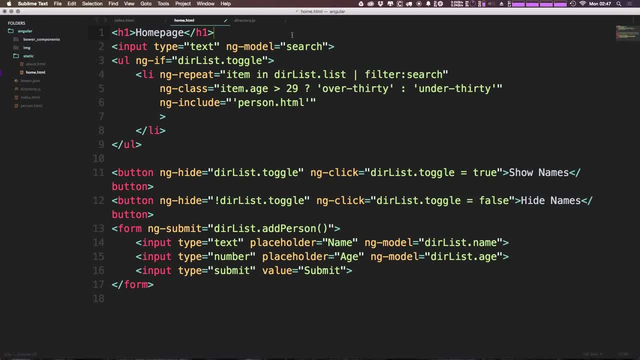 We're going to create a hello world directive And it's going to just output hello world before making this a little bit more complex and actually having a directive to contain functionality and pass in data and really just show you why you'd use them. So now I mean the Angular definition in their docs for directives says: at a high level, 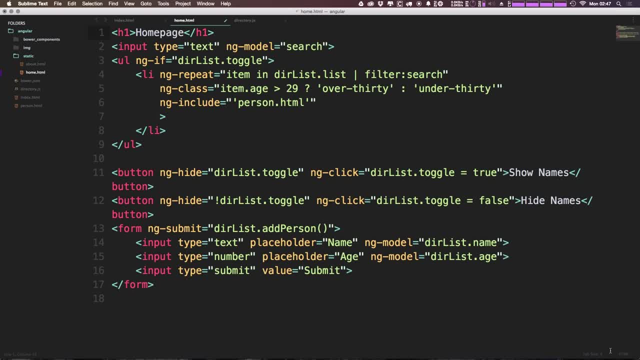 directives are markers on a DOM element that tell AngularJS, that tell AngularJS's HTML compiler to execute a directive, So that's going to be a little bit more complex, So I'm going to be going to be talking about how to attach specific behavior to that DOM element. 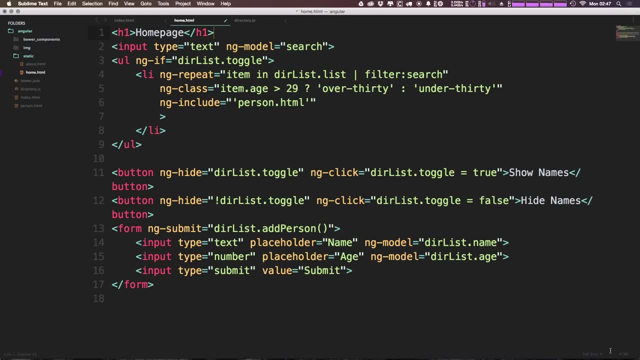 I mean, if you didn't know what a directive was after that sentence, you may still not know. It just doesn't go ahead and say it. However, what a directive is in its very most basic sort of understanding is it's almost like a web component or a web element, without it actually. 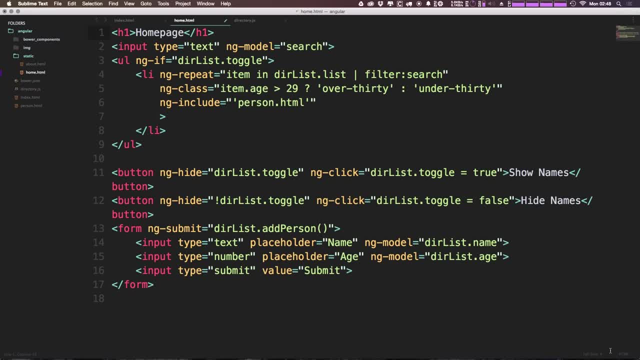 necessarily being one. So if you use something like Polymer, you've seen that you can create your own HTML elements. Now, Angular version- one at least, does not use web components. However, you can think of directives as something very, very similar. Essentially, a directive allows you to create: 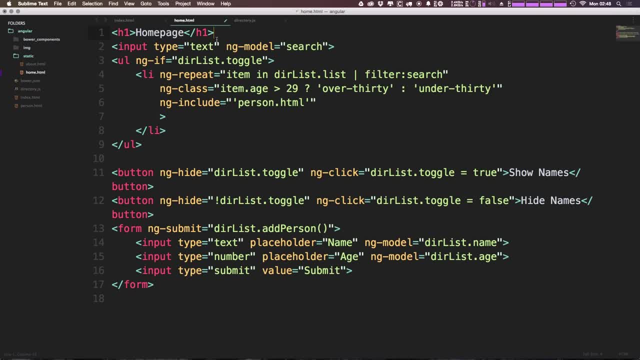 your own HTML element here And you can use that element to attach functionality and all sorts of cool stuff. Or you can just simply create a directive that is on an attribute itself instead of being its own element, And the same thing is when you use this ng. 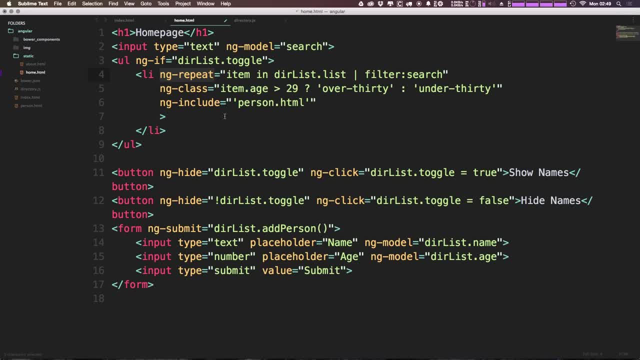 when you use this ng repeat, it's essentially telling Angular to do something. Okay, so let's go ahead and create our hello world before diving in to too much of the crazy stuff. So let's first let's just save this as is here. Let's head to our directoryjs file that we had And you can see we 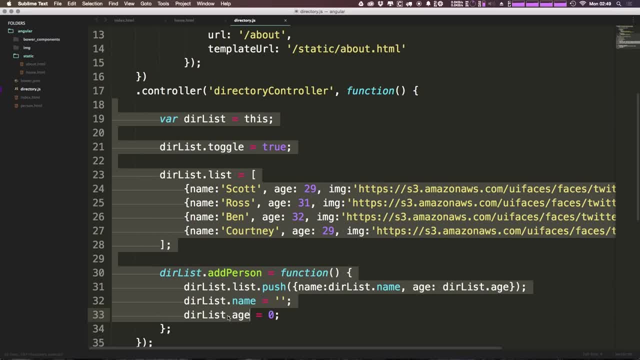 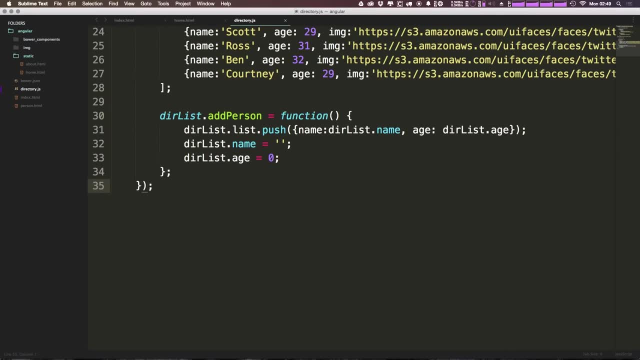 had our config, we had our controller And at the end here we just have a semicolon. Now what we can do is just save this as is here And then we can just save this as is here, And then we can just like we had dot controller here And in a larger application. you'd want to break all this. 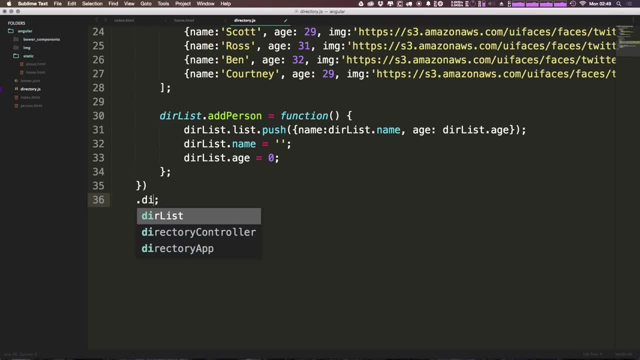 stuff out, But we can just say dot directive. Now in here we're going to give it a name Now. this name is going to be hello world, And notice how this is camel case. We're going to talk about this a little bit more in a second, But this is important. So this is going to be camel cased. 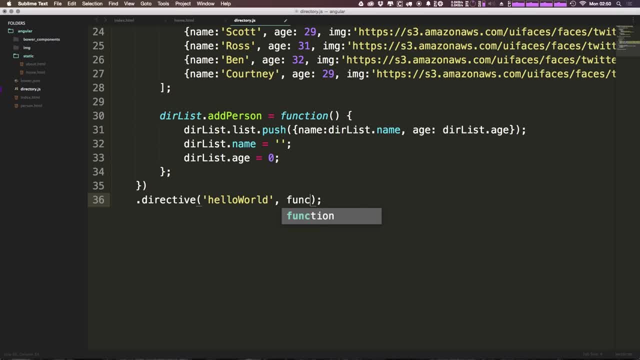 and your should be as well. So let's type in function. Okay, so now we have the contents of our directive. Inside of our directive we can just simply say return- Spell it correctly. we can say return brackets. Now let's say template. 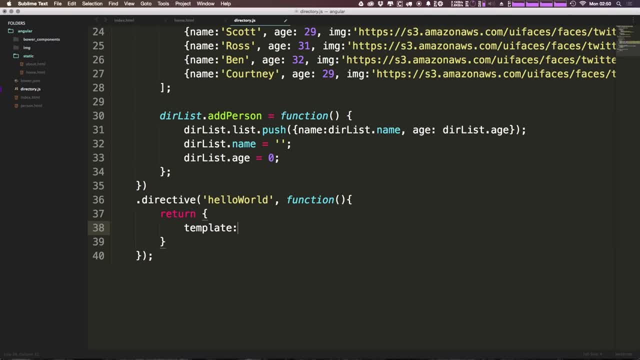 And the template is going to be, in quotes, just the words Hello world, like. so That's it At its very most basic. we're going to be able to use the Hello world directive in our application, And it's just going to simply output the text Hello world. So now we can come to our homepage. 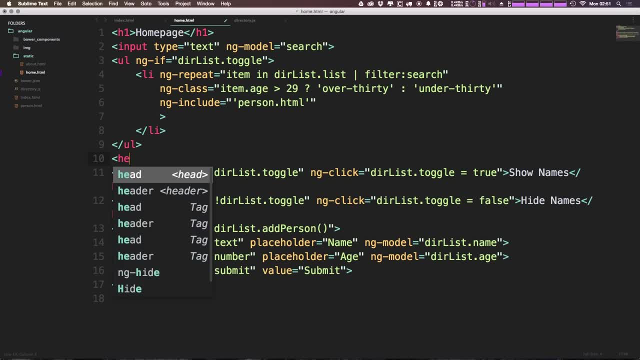 and we can say: Hello, hyphen world. So now this is where the camel case emphasis really needs to be stressed. If you'll notice, in when we're using this as an element, or even as a property on an element, we are using a hyphenated syntax. Now, this is really the way that Angular prefers you do. 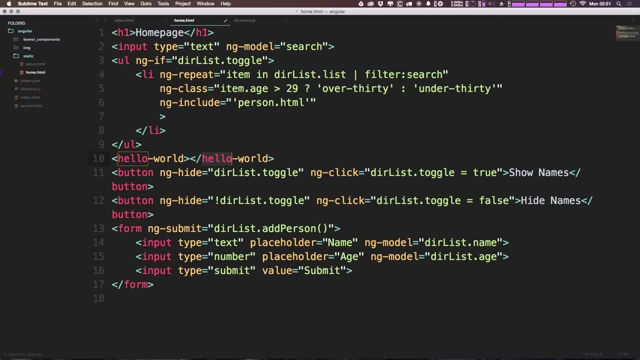 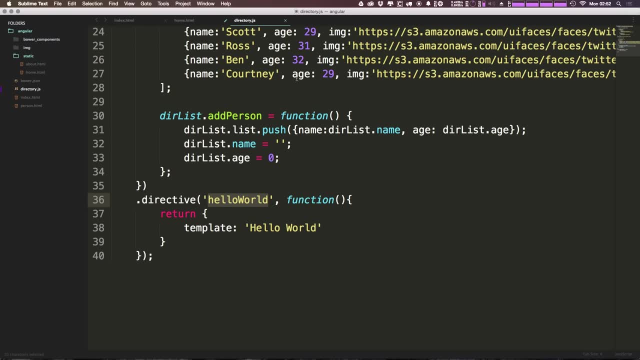 this now is to have a hyphenated word like Hello, hyphen world, and then in your directive to declare it in camel case. Now there are some rules as to what will actually work here, with this hyphenated being turned into camel case, whether or not you're actually using this syntax. However, 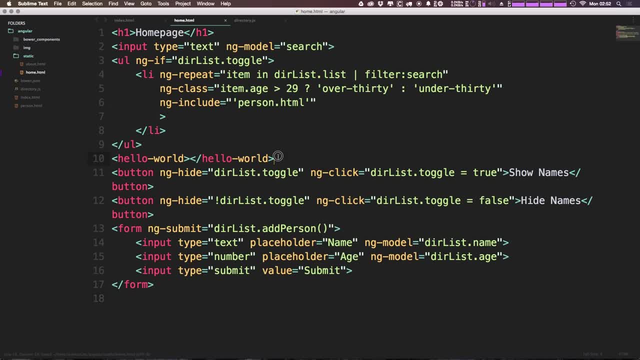 for this first example. it's important to just stress that this is this way for a reason, And you should follow these same sort of guidelines. Okay, so we have Hello world here in a camel case. we have Hello world here with a hyphen. 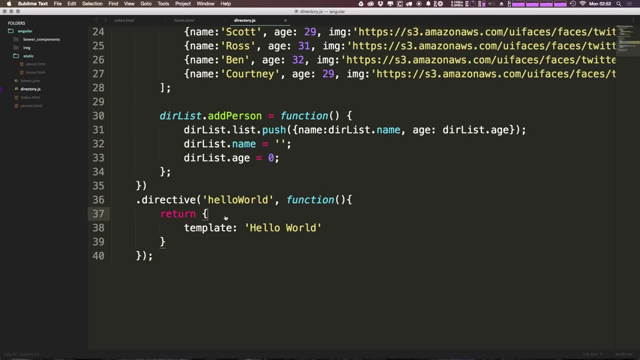 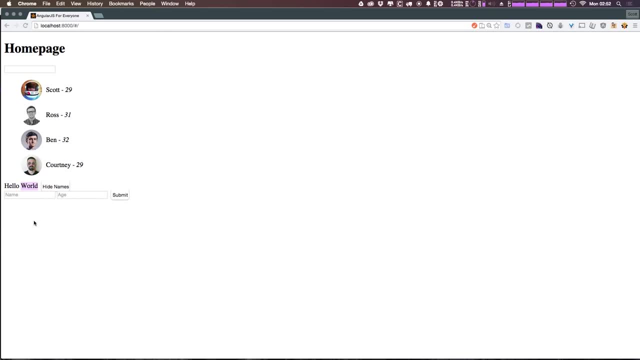 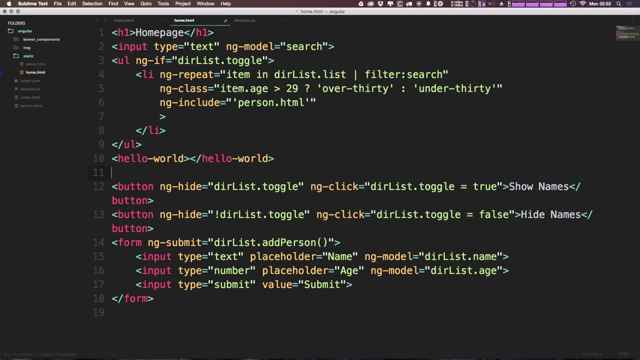 and we have Hello world here with camel case. let's come to our application, let's refresh And boom, we have Hello world sitting right here And anytime we want to go ahead and throw this Hello world directive in our application, like so, we can just. 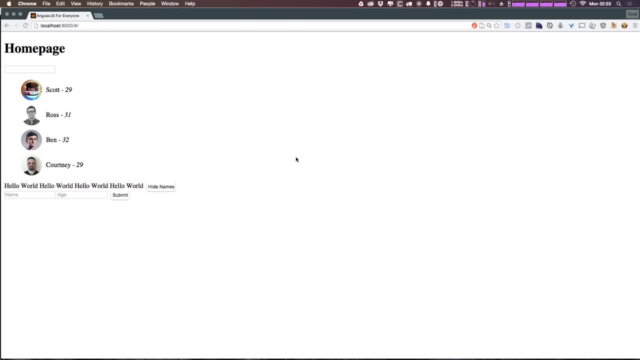 paste in here a bunch of times. every single time it's going to output: Hello world, Cool. So in the next video, we're going to be showing you a couple of more exciting, interesting things about directives, before really getting into some cool functionality. What we're going to be doing is 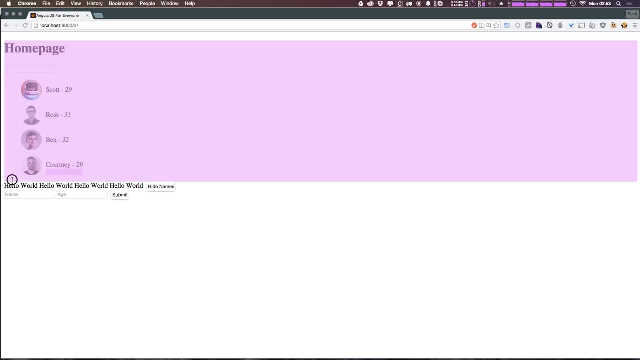 actually using the directive to have our individual person's name and age here, So check it out. we're going to get into the next video. As always, this is Scott with Level Up Tutorials. If you have comments, leave a comment in the video or hit me up at Twitter or Facebook at Level Up Tutorials. I love to hear from you. Thanks for watching and I'll see you in the next one. Bye.